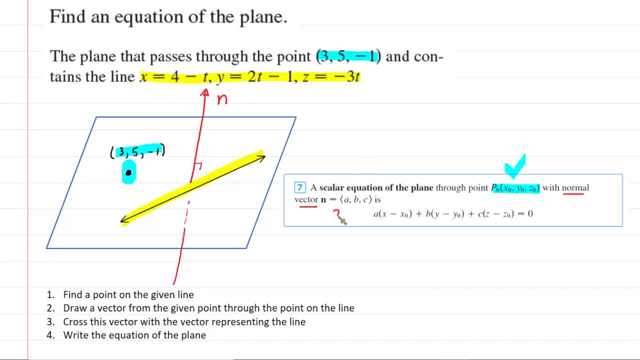 We don't have that. That's. the great challenge is to figure out what that normal vector is. Once we have the normal vector along with the given point, we just plug it into this equation for the scalar equation of a plane, and we are in business. 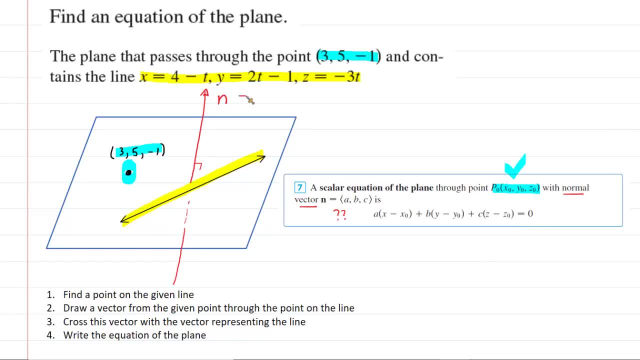 So, again, the great challenge becomes to find this normal vector right here. And so we're going to adopt a four-step strategy, and we will see why this is going to work as it sort of unfolds In the first step. what we're going to do. 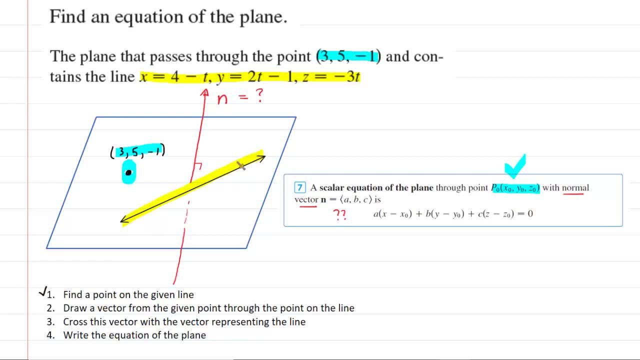 is simply find a point on this given line, which we have highlighted in yellow. You can do that by selecting any value that you want for t. You could plug in: t is equal to zero. You could plug in: t is equal to 1,000.. 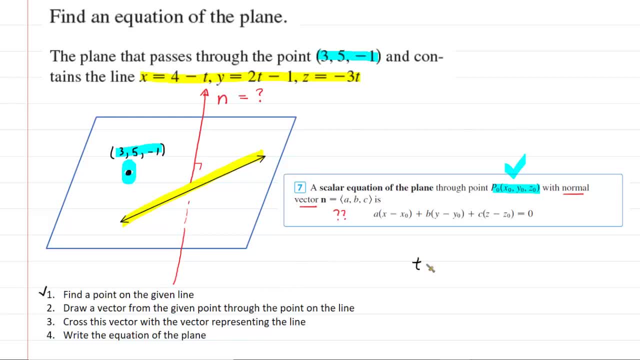 And it's going to be easy for us, of course, to make t equal to zero. So this will give us a second point that we can work with, And let's go ahead and plug zero into those parametric equations above. So x would equal four minus zero, which is four. 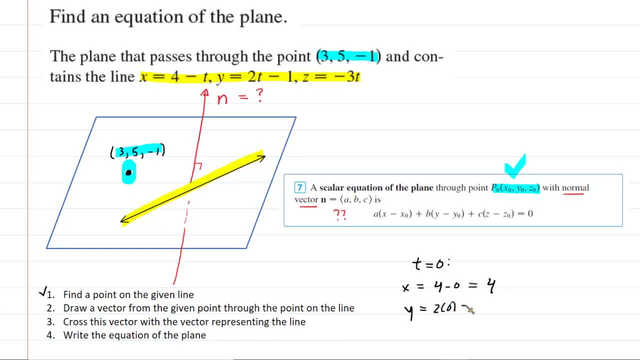 Then we have: y is equal to two times zero minus one, and that's going to give us negative one. And then z is going to equal negative three times zero, which indeed is zero. So these x, y and z coordinates right here would be: 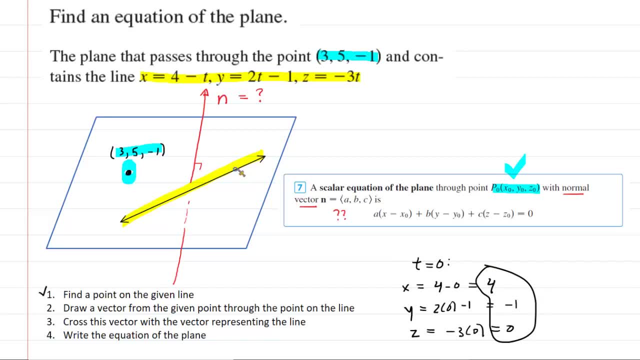 well, the point on this line. We don't have to plot it to any degree of scale or accuracy, We'll just arbitrarily put it right there. That point will be four comma negative, one comma zero. The next thing that we need to do is step two. 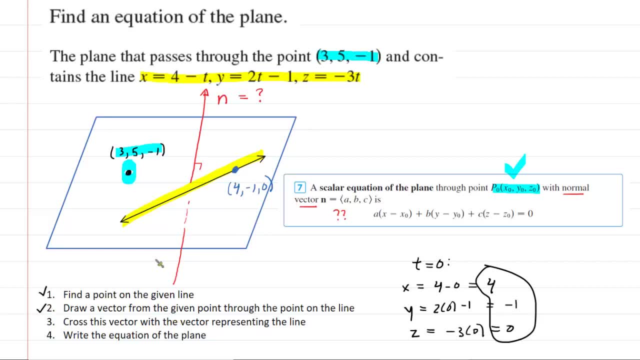 and it says to draw a vector from the given point, which is that blue one, through the point on the line. So we're just going to draw a vector originating from the given point, going through that point on the line. We will call that vector a. 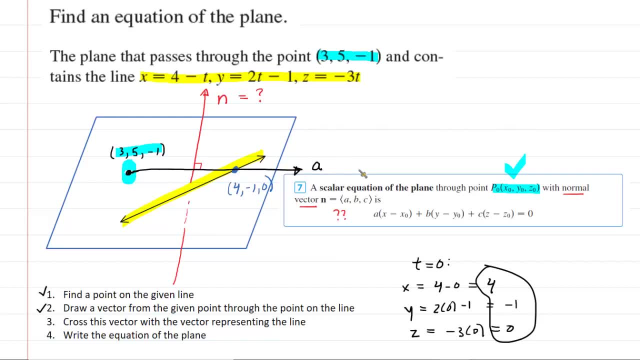 and we will need to figure out the components of that vector. And that's relatively straightforward, because you probably remember from an earlier section that to represent vector a would mean to take the difference between the x coordinates, the y coordinates and the z coordinates. 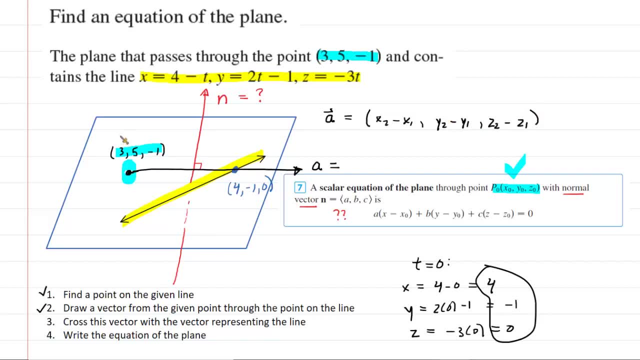 And when we're saying x, y and z coordinates, we're referring to these two points. So perhaps we could do that. So perhaps we could do that We can call this x one, y one and z one. And then this new point that we just found: 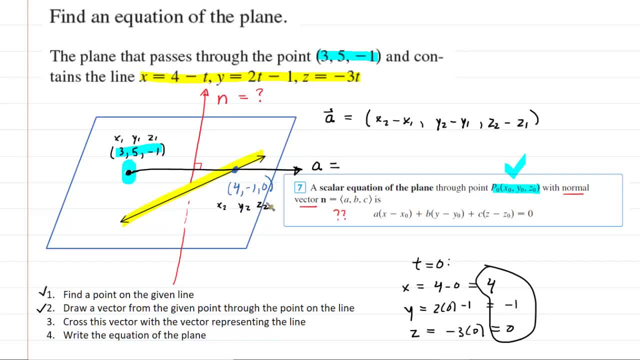 would be our x, two, y two, z, two, And again to find the vector representation for vector a, we just find the difference between the x, y, z coordinates. So make sure you subtract from the second point to the first point. 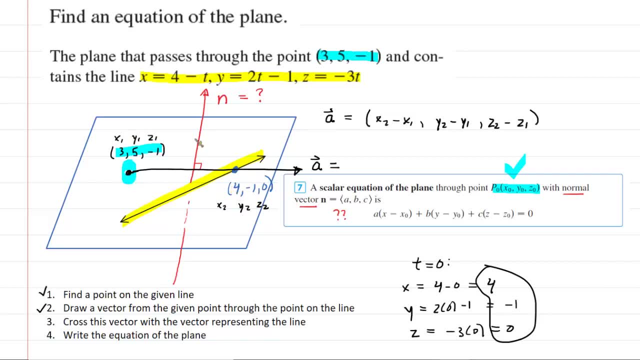 So you gotta make sure it's x two minus x one, So it's gonna be four minus three, which gives us one, And then you're gonna have negative one minus five, which is negative six, And then you're gonna have zero minus negative one. 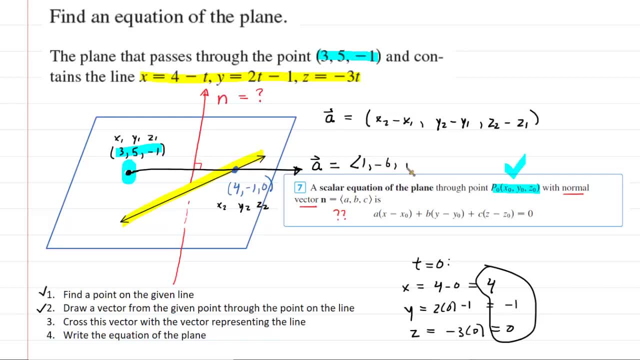 Be careful there. Zero minus negative one is zero plus one, So that's just gonna be one. So that's the vector representation of that line right there. Now we'll notice that the given line, the one in yellow, will have a vector representation as well. 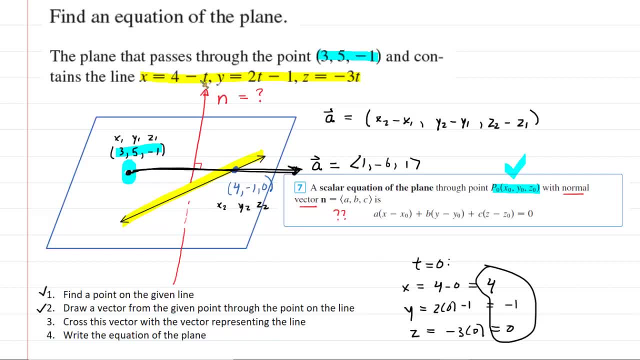 So go back to the parametric equations And what you're gonna do is look at the coefficients of the variable t. So, for example, here you have a coefficient of negative one, Over here you have a coefficient of two, And then over here it's a coefficient of negative three. 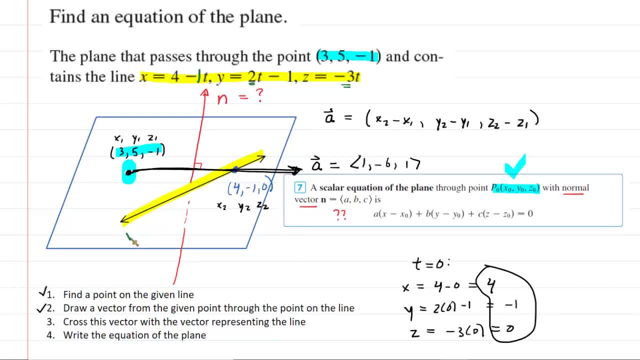 That is the vector for that yellow line. We'll call that vector b And we'll just take those coefficients again. So that's gonna be negative one, two and negative three. They're basically called direction numbers. They kind of tell us the direction and the x, y and z axis. 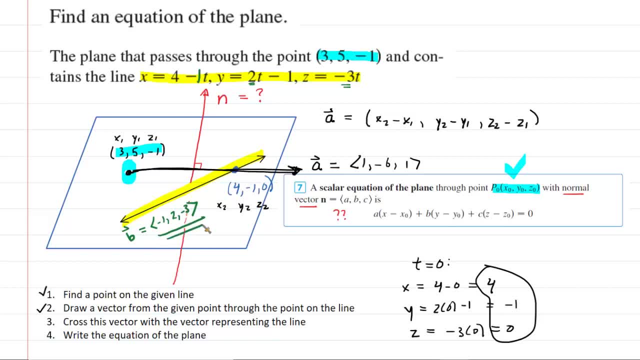 that that yellow line is moving. So this is indeed the vector for that yellow line, And then again we also have the vector for that other line that we drew. So what we will now do is cross the vector that we figured out. we called it vector a. 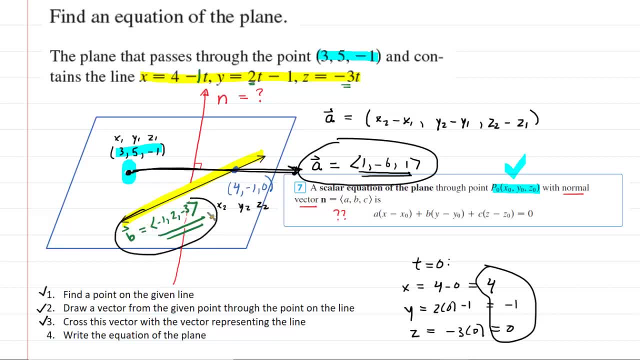 with the vector representing the line, which was vector b. And here's the beautiful thing: When we cross this vector here, vector a with the vector representing the line, we will automatically get that normal vector. Perhaps I can draw it in a different position. 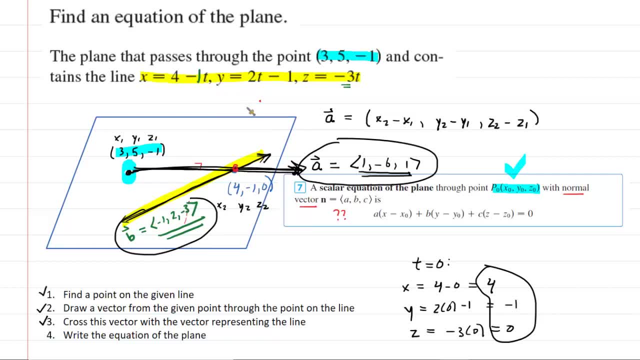 to show you what we're talking about. So right where those lines are, we're gonna draw a line. So right where those lines are, we're gonna draw a line. And when those lines would sort of intersect, we would get a normal vector once we cross them together. 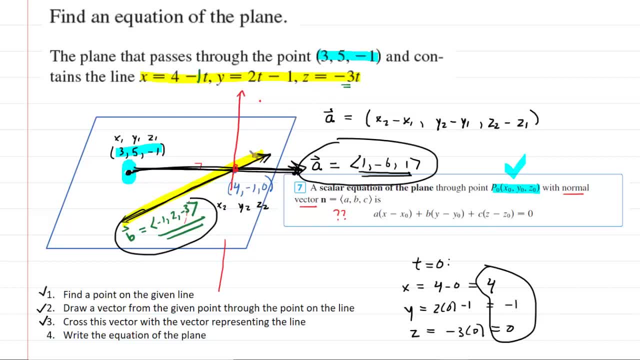 So anytime you cross two vectors, you're going to get a third vector that runs perpendicular to the original vectors. So that means that this third vector, this normal vector, would run perpendicular to the plane as well, because vector a and vector b lie on the plane. 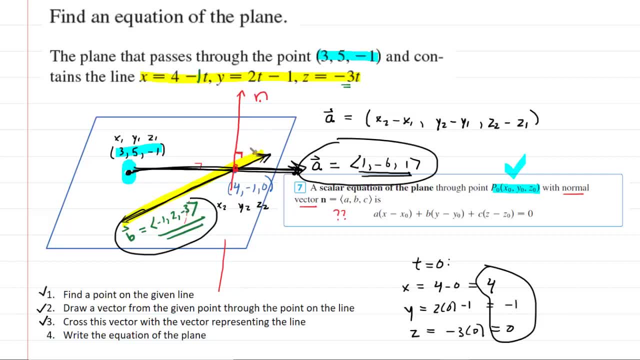 So when we cross them, that normal vector will indeed be perpendicular to the plane. So that's the key, right there. Really, step three is the most important here, And so we're going to go and we're going to cross them. So this is a whole little problem in and of itself. 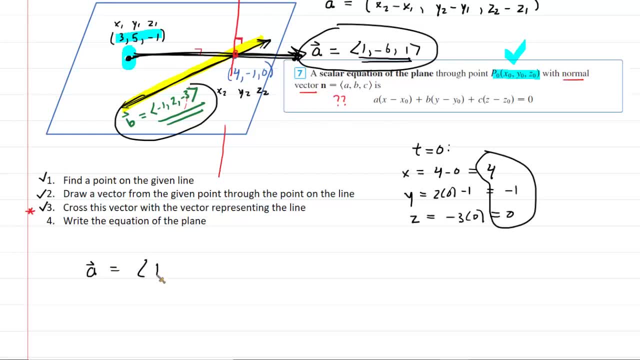 So let's just rewrite the vectors We have. vector A is 1, negative 6, and 1.. And then vector B is equal to negative 1,, 2, and negative 3.. And again we're going to find the cross product. 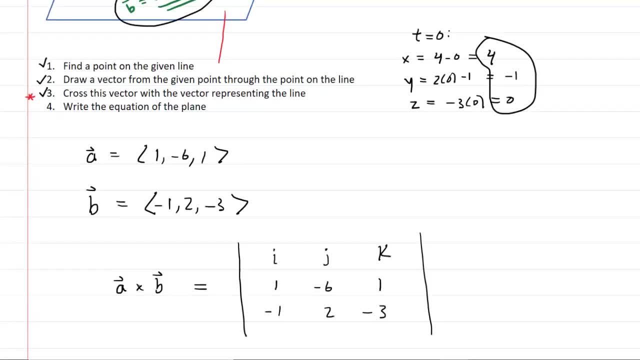 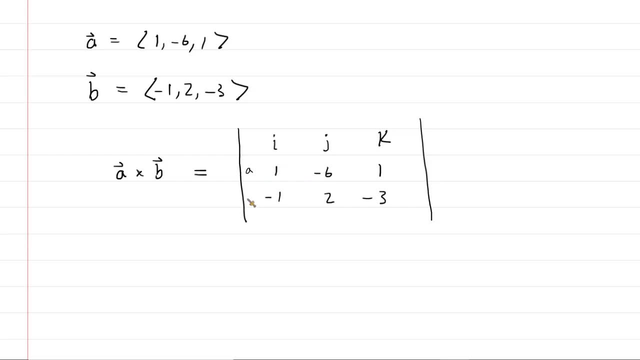 Let's take a look at that. Okay, so here is the setup for the cross product. We basically just put sort of the X, Y, Z components of each vector horizontally- This is vector A, This is vector B- And to do the cross product whoopsies we're going to have to basically do some determinants. 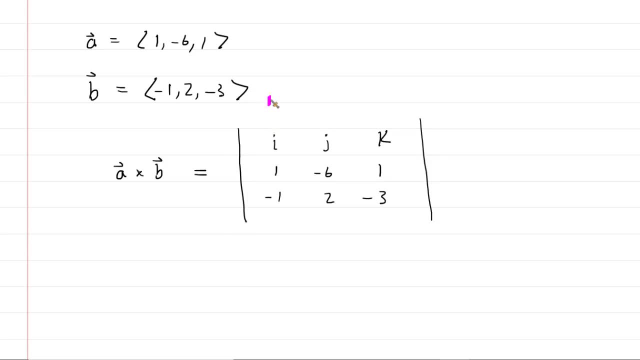 So, for example, when we do the cross product, the first thing you want to do is cover up the I column And that leaves you with a 2 by 2 sort of matrix, And you're going to want to find the determinant of that little 2 by 2 matrix. 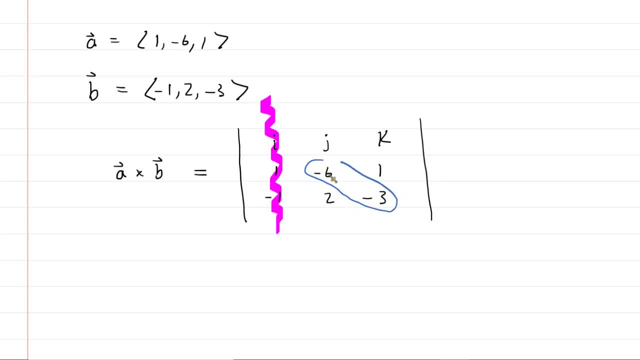 And that's pretty easy. What you do is you just sort of cross multiply. You do those two numbers multiplied, So you're going to get Obviously 18.. And then you're going to also multiply those two numbers, which gives you 2.. 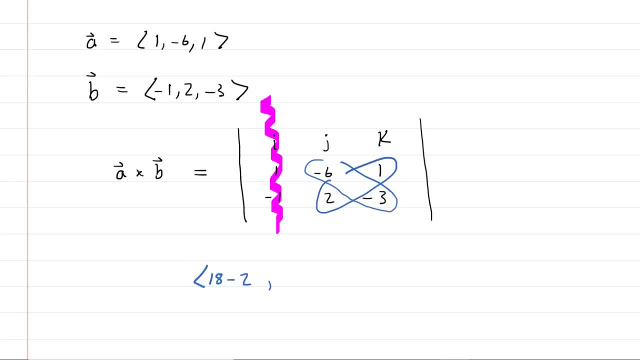 And then you simply subtract them. So that would be sort of the first result of our cross product for the I hat direction or the X direction, For the Y or the J hat direction. what you're going to do is cover that column up. 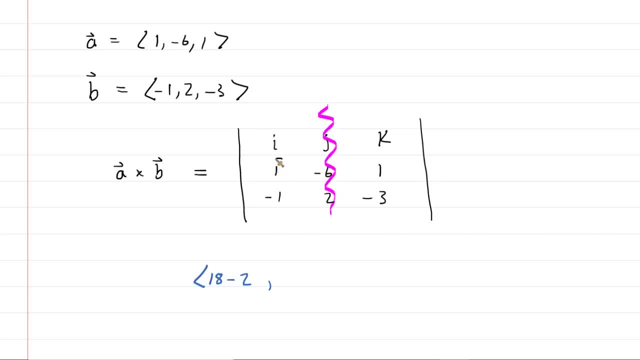 That's going to give you a different 2 by 2 matrix. Again, you do the determinant. So you're going to do 1 times negative 3, which is negative, 3.. And then you're going to do negative 1 times 1,, which is negative. 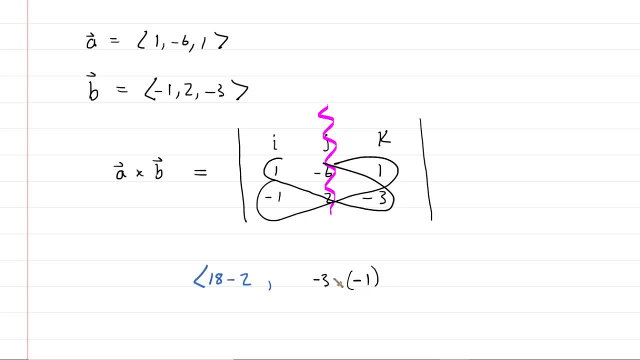 And then you're going to subtract them. Also- and this is really important for this middle component, this sort of Y component, make sure you negate the result. That's very important. Don't forget that negative sign right there. That is crucial. 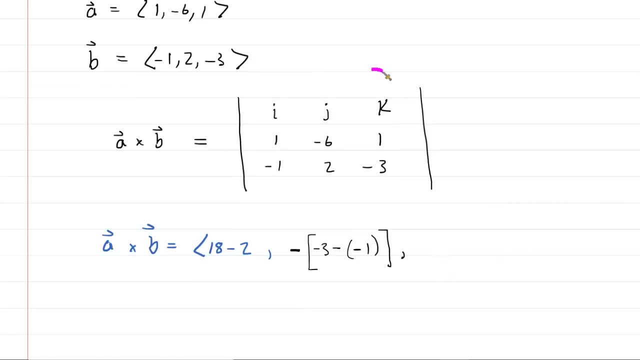 And then to get our Z component, we're going to kind of cross off the K hat column right here and do one more determinant. We're going to have 1 times 2, which is 2, minus negative 1 by negative 6, which is positive 6.. 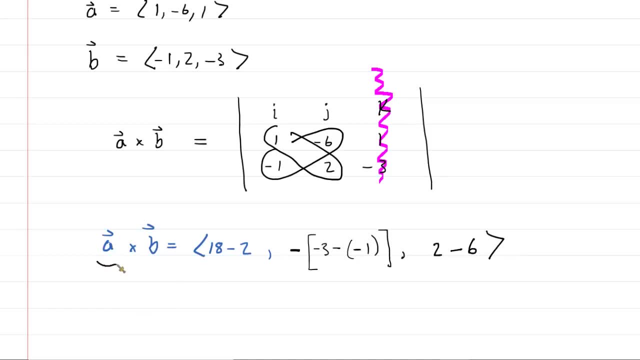 So now all we have To do is clean this up. Now, remember, the cross product between those two vectors gives us a third vector that is perpendicular to both of those vectors, which is indeed perpendicular to the plane. So therefore it's the normal vector. 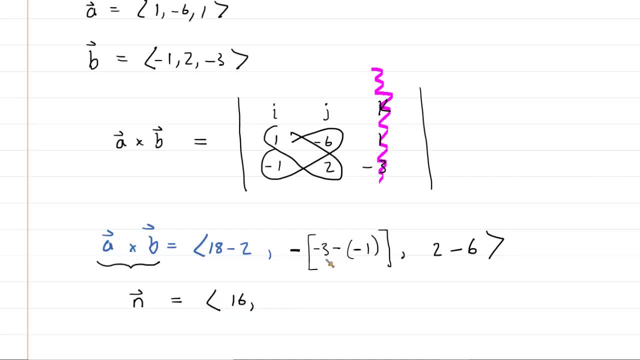 We simplify, We get 16.. Let's see: Negative: 3 plus 1 is negative 2, but then negate that, So you get positive 2. And then 2 minus 6 is negative 4.. So there's your normal vector. 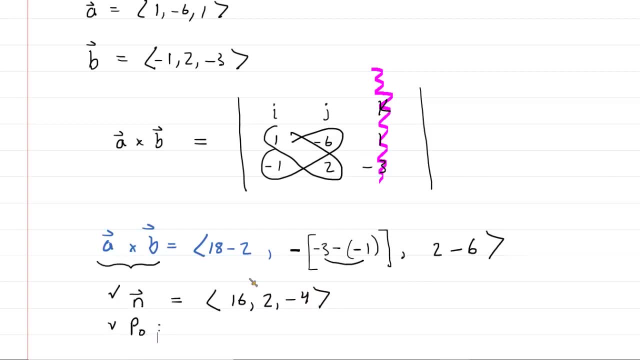 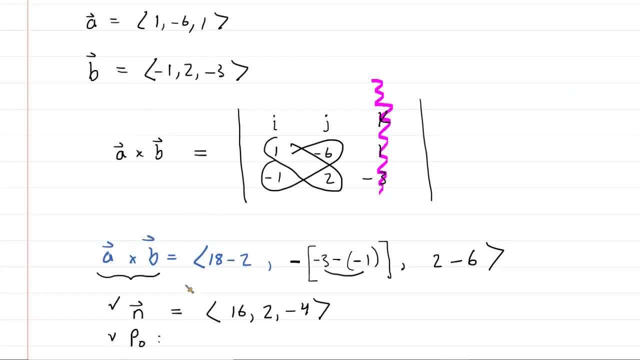 We also had a point on the plane. We can call that P naught And if we go back up we recall that P naught Had the coordinates of 3, 5, negative 1.. 3, 5, negative 1 are the coordinates. 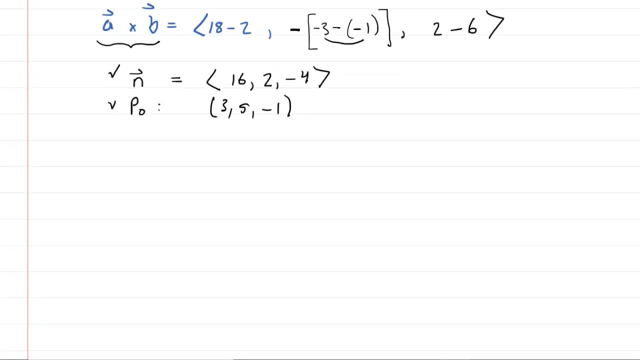 And now we revisit the equation of a plane, the scalar equation, There. it is right there, And we can just label things again here to keep it straight. The point is going to be our X naught, Y naught, Z naught. 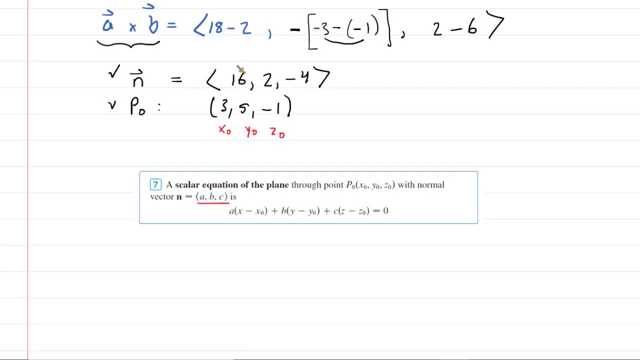 And then the normal vector will have these sort of direction numbers here: little a, little b, little c, And we just plug them in. So here we go. We're going to have our little a of 16 times X minus our X. 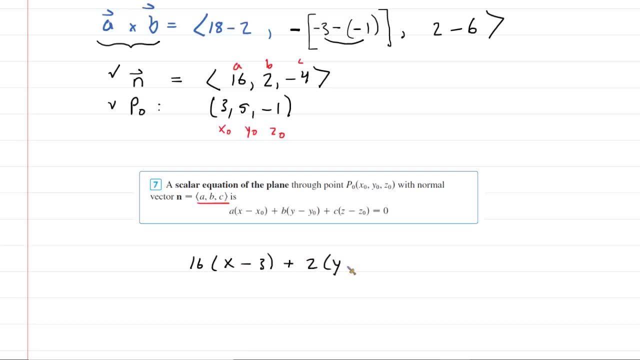 X naught plus our little b, times Y minus our Y naught, And then plus little c, That's going to be a minus 4.. Be careful, there Times Z minus negative 1. So that will become plus 1 equals 0.. 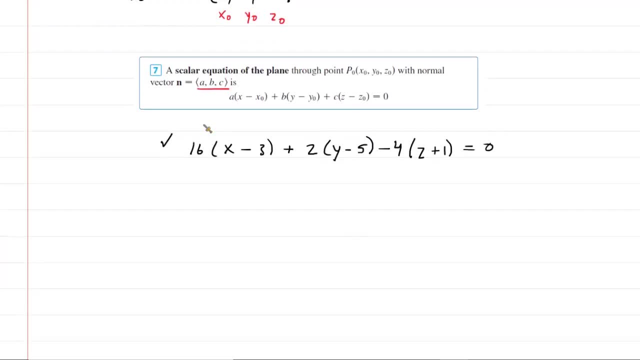 And that's perfectly fine. Your professor might accept that as a final answer. But we can do a little bit better by distributing all of these direction numbers here. So we're going to have 16X minus 48 plus 2Y minus 10.. 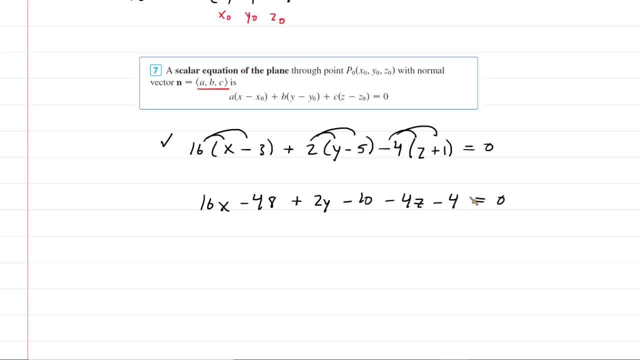 Minus 4Z minus 4 equals 0. Then we can combine all the constants, So here here and here. So negative 48 minus 10 minus 4 is negative 62. And then you can add that 62 over.